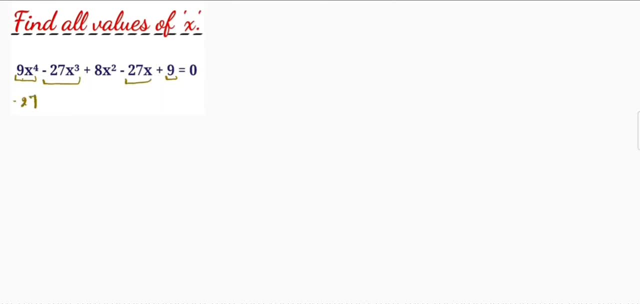 they are also same. they are 27.. So these type of equations are known as reciprocal equation. Why do we call them reciprocal equations? Because when we change x to 1 upon x in these equations they will be equal to 0. So if we see the coefficient of x raised to power 3 and x raised to power 3, 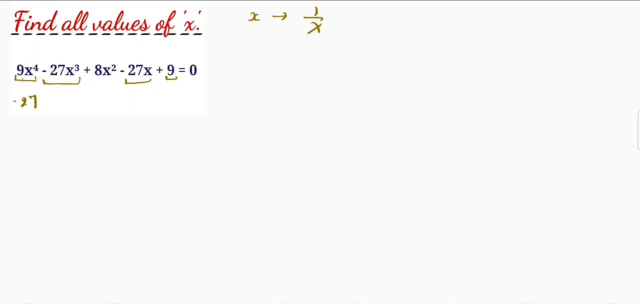 won't change means they will remain same. Let's see how, instead of x, I will take 1 upon x, So this will become 9, 1 upon x, raised to power, 4 minus 27, 1 upon x, raised to power, 3 plus 8 upon x square. 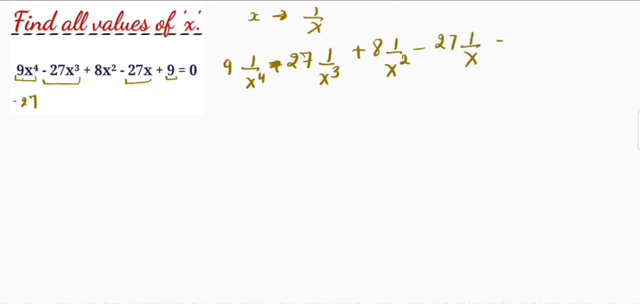 minus 27, 1 upon x plus 9 is equal to 0, as I have changed x to 1 upon x, Now I will take the LCM equation. So this will be x raised to power 4.. So first I will get here 9, then I will get 27 plus 8 x square. 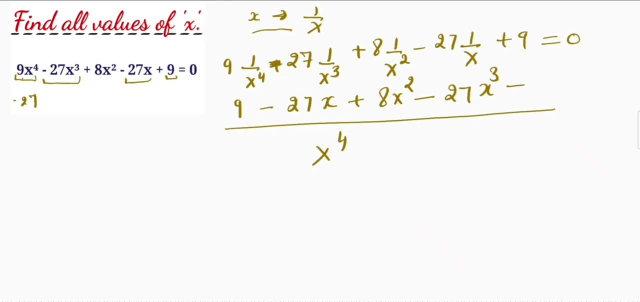 I will get minus 27 x raised to power 3 plus 9 x raised to power 4 is equal to 0.. Now we know that x raised to power 4 cannot be equal to 0. it means 9 minus 27 x plus 8 x square, minus 27 x raised to. 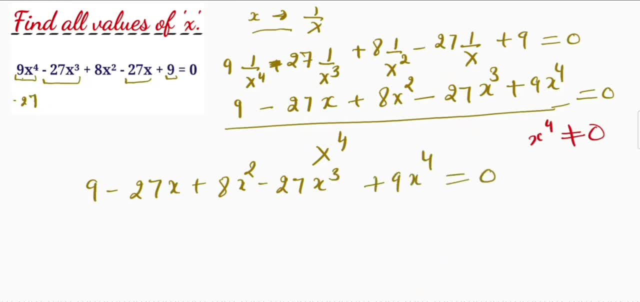 power 3.. So this will be 9, 1 upon next, 1 upon 3 plus x. I will subtract it so that this equation becomes 9 x raise to power 3 plus 9 x raised to power 4 plus 9 x raised to power 4 is equal to: 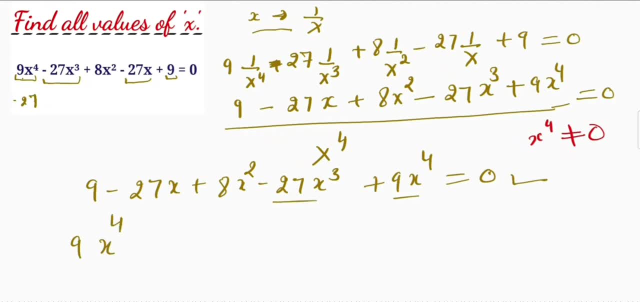 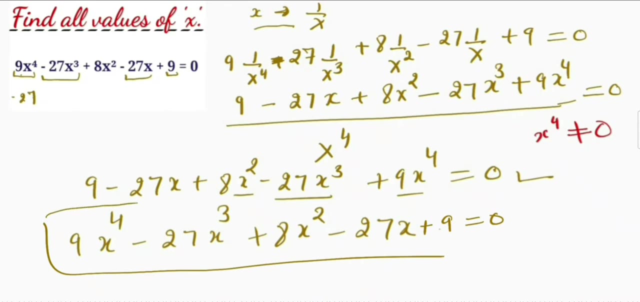 0.. Now I can write this equation in standard form as: so: this 9 x raised to power 4 will come first, and then negative 27 x raised to power 3, after that, plus 8 x square, then negative 27 x equals 9, which is equal to 0.. If I see this equation- and this equation is my original- 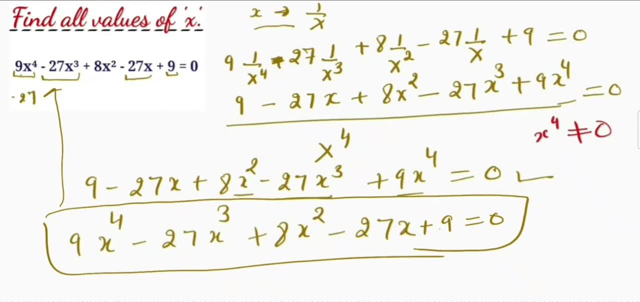 equation. So I am finished here, So let me compute this Mitar twisted linear dah Professions. so when you compute, So these type of equation where when we replace x to 1 upon x, they won't change, they are known as reciprocal equations. Now let's see how we can solve these type of the reciprocal equations. 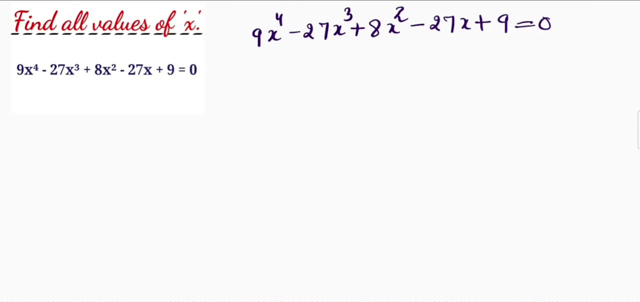 step by step. First step which I am going to take: f1: divide this whole equation with x square, So we will get 9 x raised to power 4 divided by x square, minus 27 x raised to power. 3 divided by x square plus 8 x square upon x square, negative 27 x upon x square plus 9 x square is equal to: 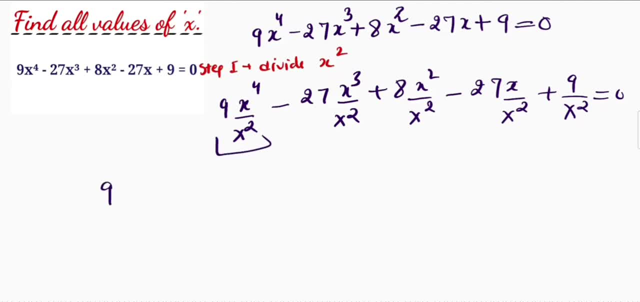 0.. So this will become 9 x raised to power 4 minus 2, which is x square minus 27. this will become 9 x raised to power 4 minus 2, which is x square minus 27. this will become 9 x raised to. 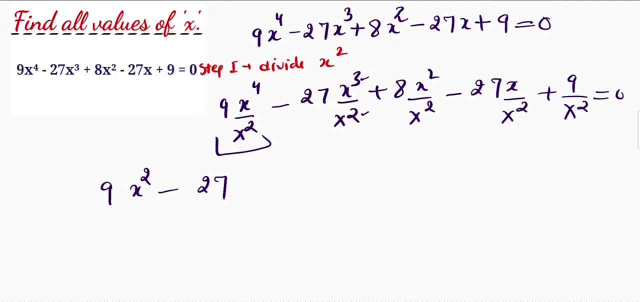 power 4 minus 2, which is x square minus 27, this will become 9 x raised to power 4 minus 2, which is come x raised to power 3 minus 2, which will be x plus. this will get cancelled with this 8 negative. 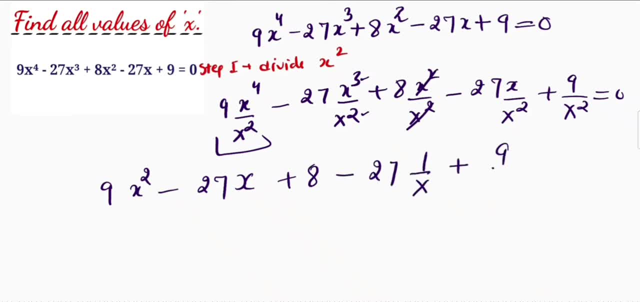 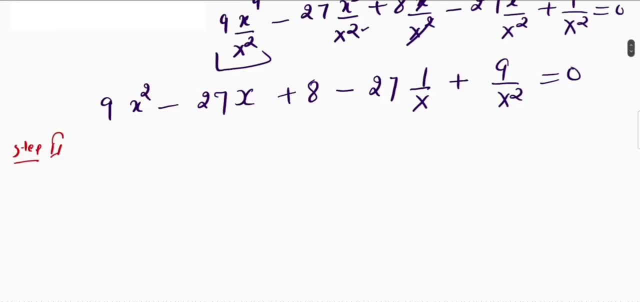 27, 1 upon x plus 9 upon x square is equal to 0. so second step: we have to rearrange all these terms. so first i will take this 9 x square and plus 9 divided by x square together, so i can write. 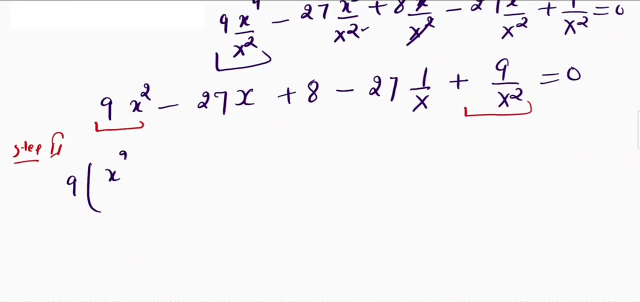 this as 9. i can take common from this with x square plus 1 upon x square. so second, i will take this negative 27 x and negative 27, 1 upon x together, so i can take this 27 out and inside i will be left with x plus 1 upon x and this 8 will come last. so next step is step 3. here i'll take 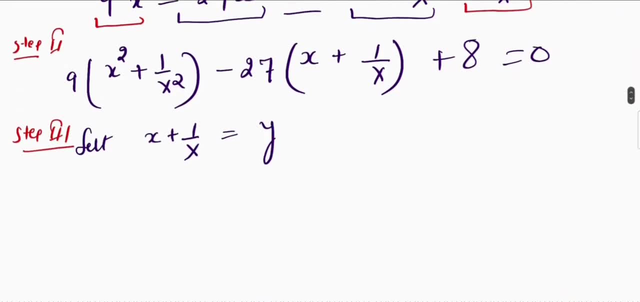 this: let this x. x plus 1 upon x is equal to y. I can use this identity that x square plus 1 upon x square is equal to y square minus 2.. So here I have used this identity: a square plus b square is equal to. 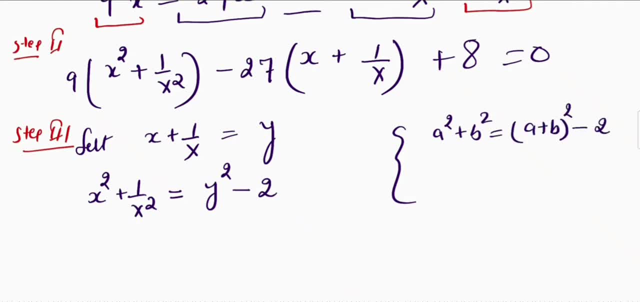 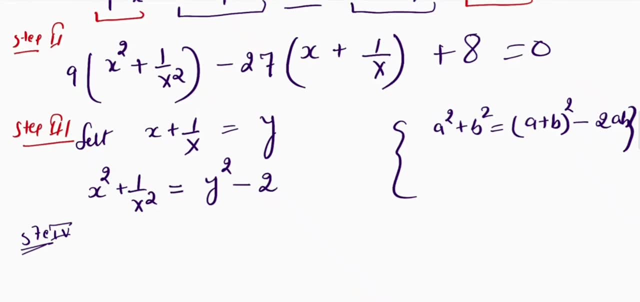 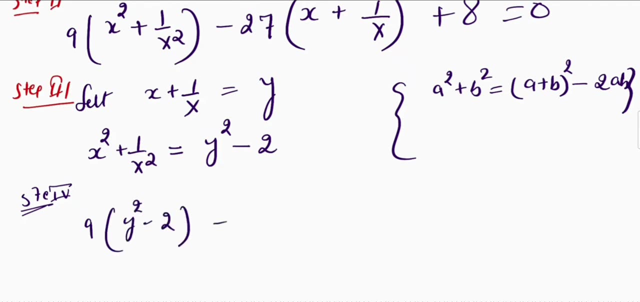 a plus b, whole square minus 2ab. In fourth step I will put all these values in the equation which I have got in step 2.. I can write this as x- sorry- 9 into y. square minus 2 minus 27y plus 8 is equal. 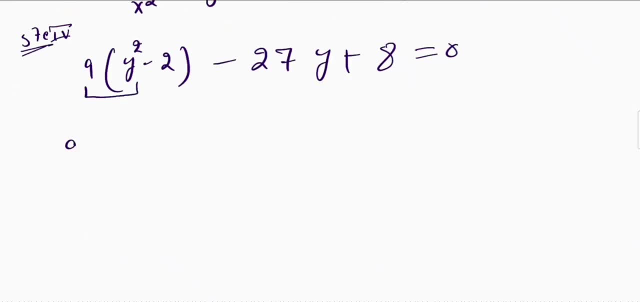 to 0.. So let me open this. I will multiply 9 inside, So this will look like 9y square minus now again, 9 with 2 negative 18 minus 27y plus 8 is equal to 0. So this will become 9y square. 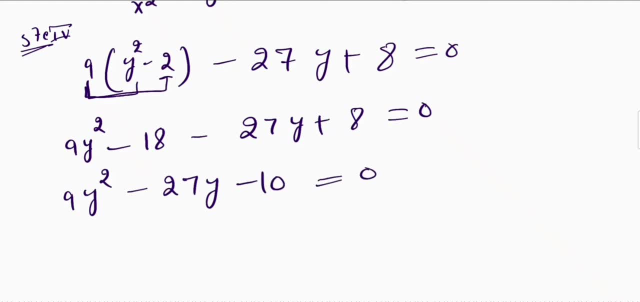 minus 2.. 27y minus 10 is equal to 0.. Now this is my quadratic equation. Now let's find the rules of this quadratic equation. I will use here midterm split method. So 9 into 10 is 90.. So factors of: 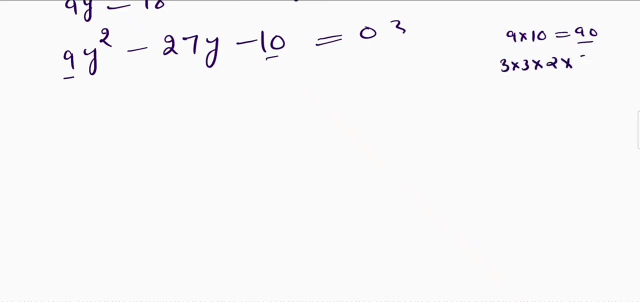 9 are 3 into 3, into 2 into 5.. So if I rearrange I will get that 15 into 2, 30 and 3.. So I will take negative 27 with these two numbers. like I can split this as negative 30y and 3y, Let's see I can. 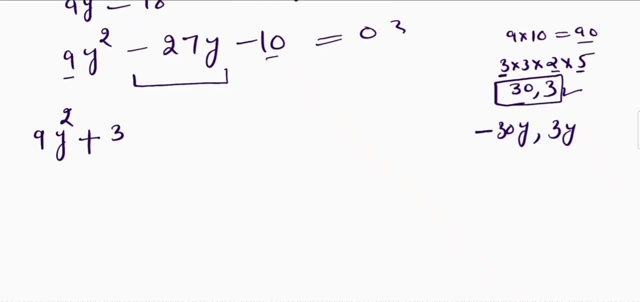 put this here. So 9y square minus plus 3y- I will take here- and then negative 30y minus 10 is equal to 0.. If I add these two, I will get negative 27. So I will take these two terms together and these: 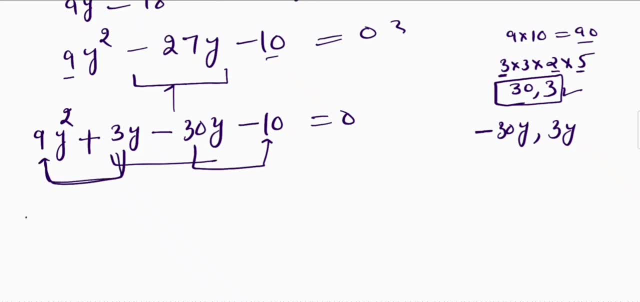 two terms together. So from these two terms I will get negative 27.. So I will take these two terms. I can take 3 and y out and inside. I will be left with 3y plus 1, and from these two terms I can take: 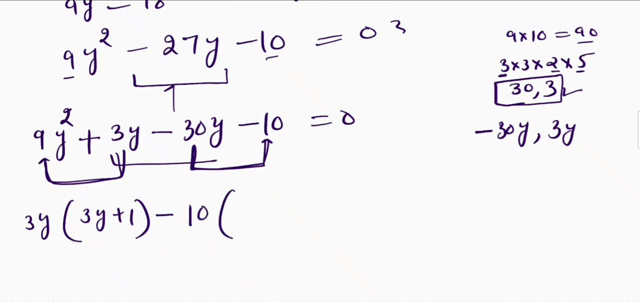 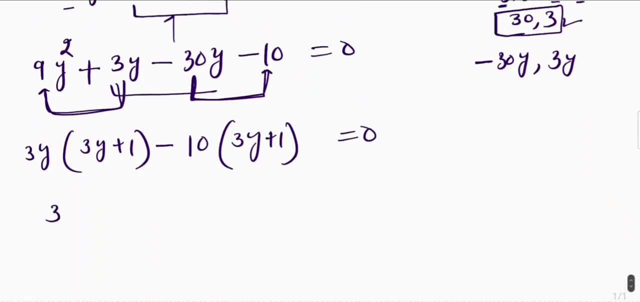 this minus out and 10.. So inside I will be left with: 3y plus 1 equals to 0. So here I will get two values of y. So this is 3y plus 1 is common, and this 3y minus 10 is equal to 0. So it means: 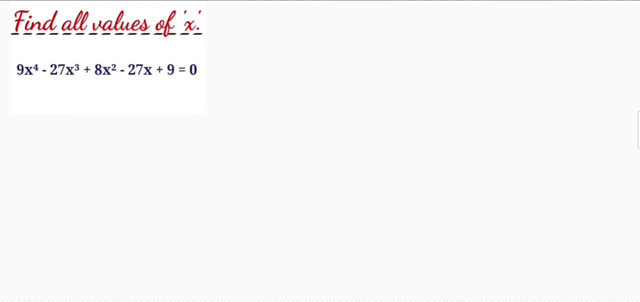 3y plus 1 is equal to 0, or 3y minus 10 is equals to 0.. So from here I will get: y is equal to negative 1 by 3, and from here I will get: y is equal to 10 by 3.. We know we have taken that x plus 1 upon x. 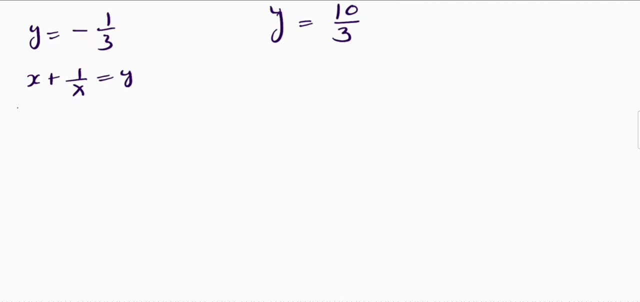 is equal to y. So first I will put: y is equal to negative 1 by 3 in this. So I will get x plus 1. x is equal to negative 1 by 3.. So I will solve this. I will get again. I will get one quadratic. 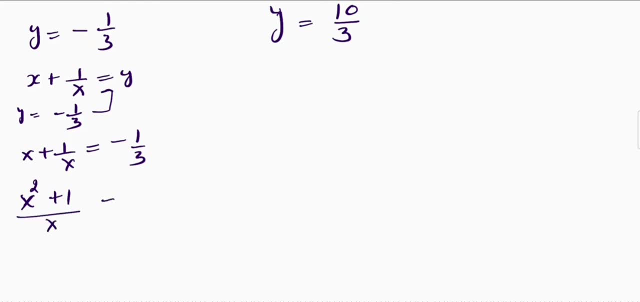 equation: x square plus 1 upon x minus 1 by 3.. So I will cross multiply them- Let me know how to do this- will become 3x square plus 3 is equal to negative x. So now I will take this x to left. 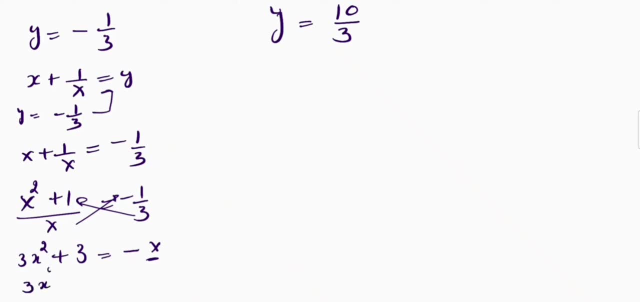 hand side of my equation, So this will become x is 3x square plus x plus 3x, So this will become 3 is equal to 0.. So now this is my quadratic equation. So here I won't be able to solve this. 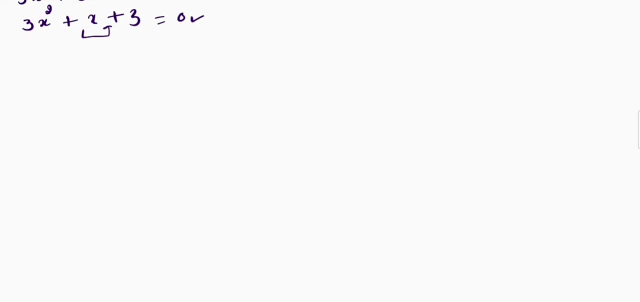 equation with the midterm split method. So I am going to use that quadratic formula to solve this equation or to get the values of x. Now the standard quadratic equation is: ax square plus px plus c is equal to 0.. If I compare this standard equation with my quadratic equation, 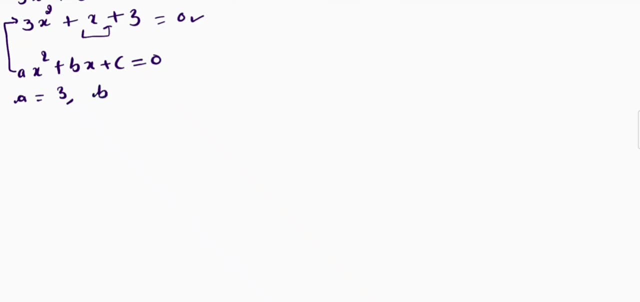 then I will find that a is equal to 3, b is equal to 1 and c is equal to 3.. So I will apply this formula: that x is equal to minus b plus minus square root of b, square minus 4ac divided by 2a. 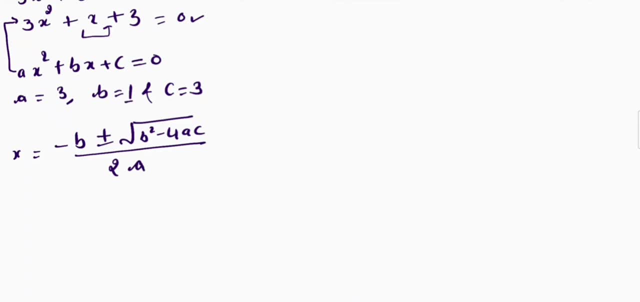 Now I will put all the values of a, b and c in this formula, So I will get negative. b is 1 plus minus square root of b, So this is 1 minus 4a is 3 and c is 3 divided by 2 into a, which is equal to 3.. So I will get here: 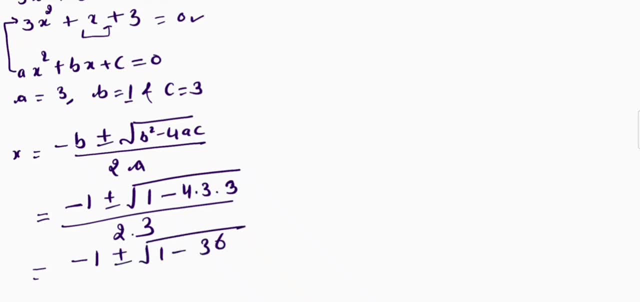 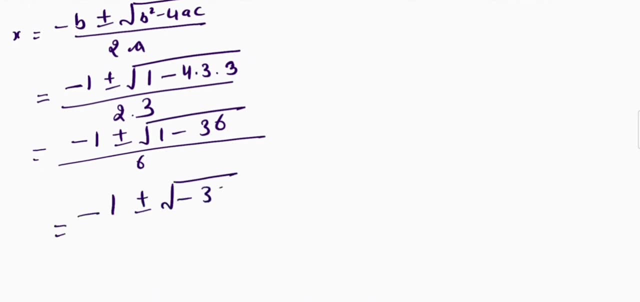 negative 1 plus minus 1 minus 36 divided by 6.. So this will become equal to negative 1 plus minus square root of negative 35 divided by 6.. So these are two values of x which I have got from my quadratic equation. 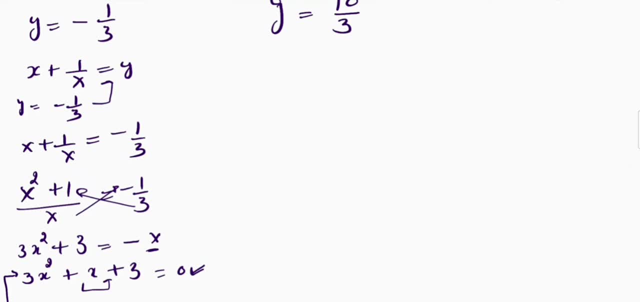 Now I will put the value of y is equal to 10 by 3 in this equation. So I will get x plus 1 upon x is equal to 10 by 3.. Again, I will take LCM, So I will get x square plus 1 divided by x is equal to. 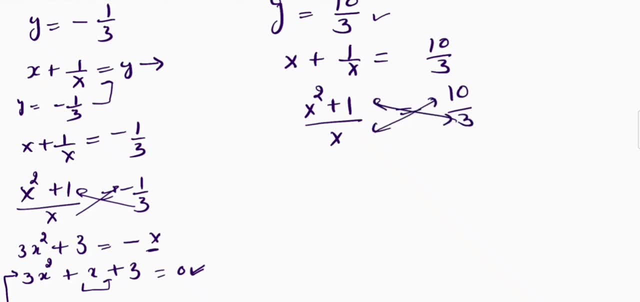 10 by 3.. So now I will cross multiply. I will get: 3x square plus 3 is equal to 10x. Now I will take this 10x to left hand side of my equation, So I will get 3x square negative. 10x plus 3 is equal to 0.. Now this is my quadratic equation and 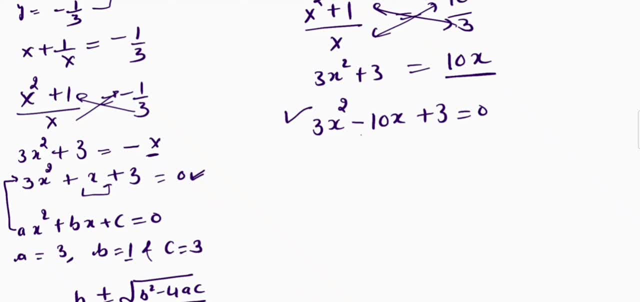 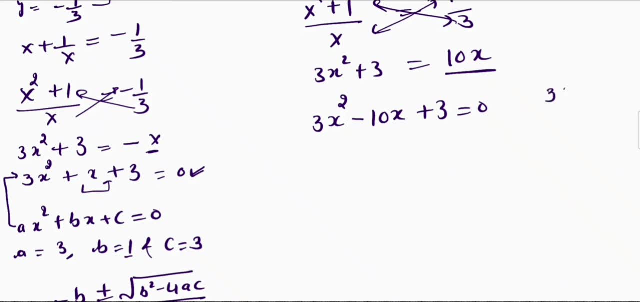 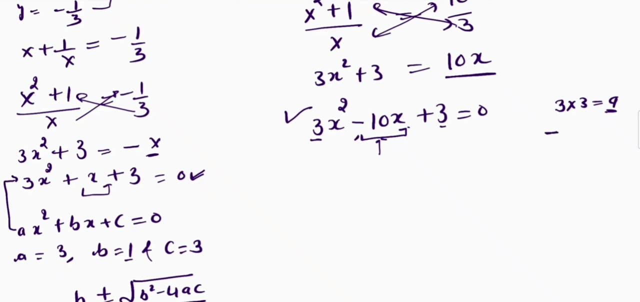 I will be able to solve this quadratic equation with midterm split method. If I multiply the coefficient of x square, which is 3, with constant term, which is 3,, I will get 9.. Now I have to rearrange this negative 10.. So I can write this negative 10 as 9 and negative 1.. So if I 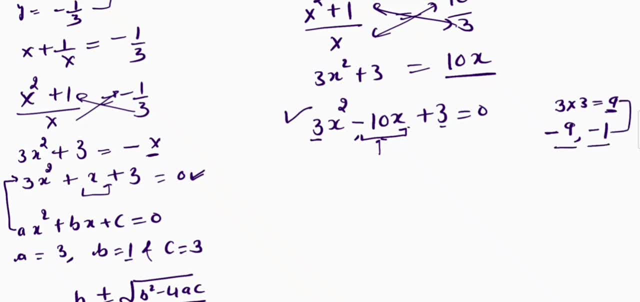 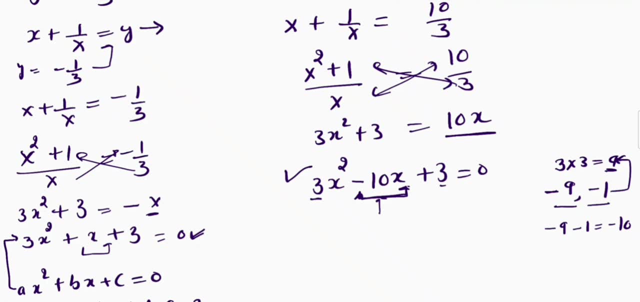 multiply negative 9 with negative 1,, I will get 9.. And if I add negative 9 and negative 1,, I will get negative 10.. So now I can write this middle term 10x, as So this will become 3x square negative 9x. 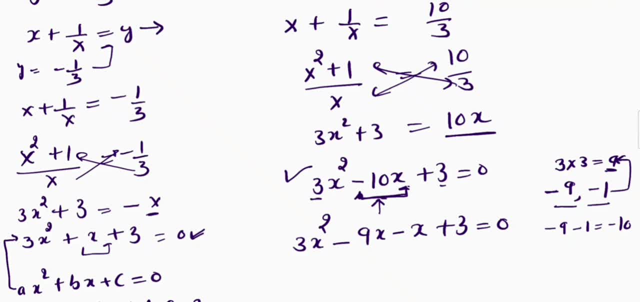 negative. x plus 3 is equal to 0.. Now I will take these two terms together and these two terms together. So from these two terms I will get 3x. square plus 3 is equal to 0.. So I will get 3x. 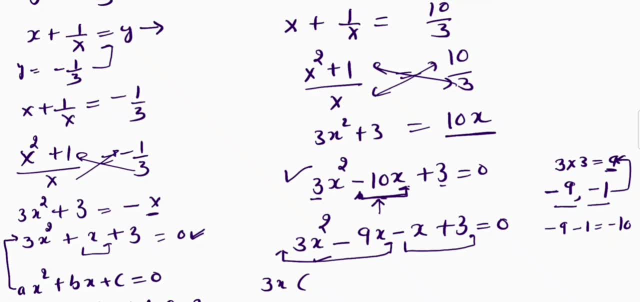 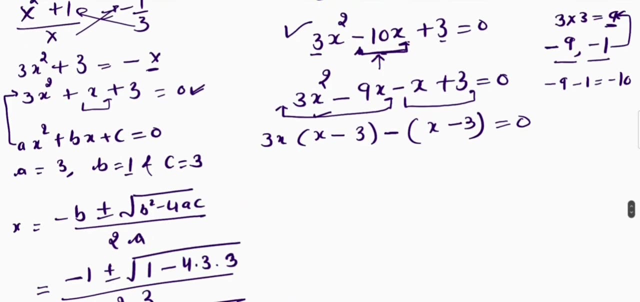 common. I will take this out. So inside I will be left with x minus 3.. And from here I will take negative out. So here I will be left with x minus 3, which is equal to 0. So this will become 3x. 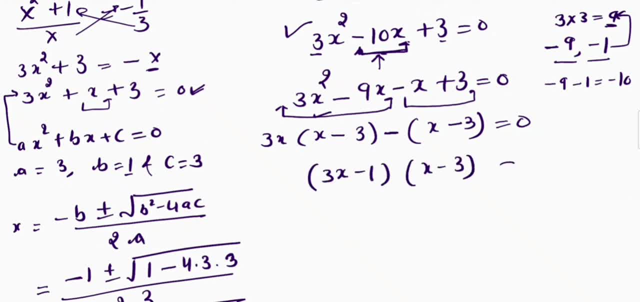 minus 1 into x minus 3 is equal to 0. So I can say that either 3x minus 1 is equal to 0 or x minus 3 is equal to 0. So from this I will get: x is equal to 1 by 3. And from here I will get x is. 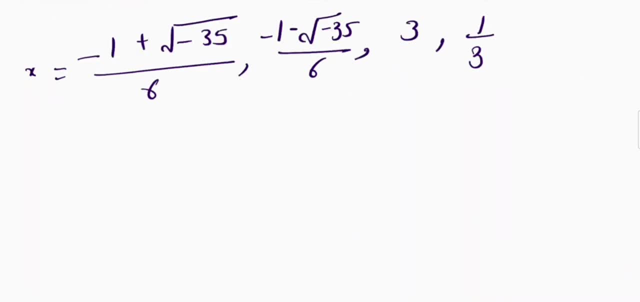 equal to 3.. So four values of given equation are negative 1 plus square root of negative 35 divided by 6, negative 1, negative square root of 35 divided by 6, 3 and 1 by 3.. If you like the video,